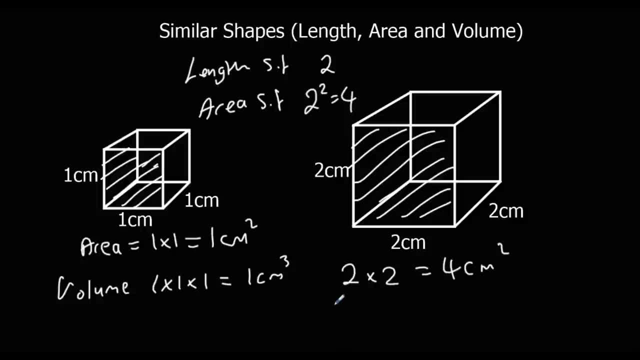 be 1 centimetre cubed And the volume for this shape would be 2 times 2 times 2.. So it's 2, which is 8 centimetres cubed. So the scale factor for volume: volume scale. 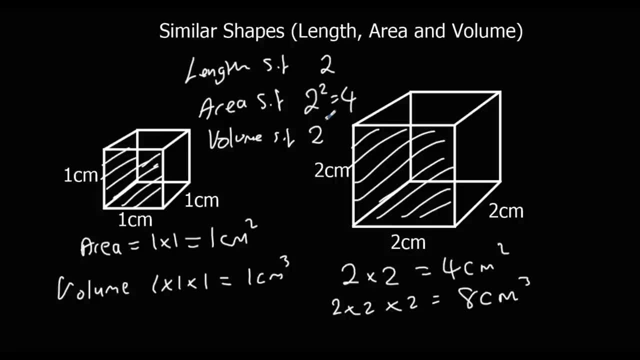 factor is times. it's 2 cubed, which is 8.. So the scale factor for area is squared and the scale factor for volume is cubed. So when you've got your normal scale factor, if you want to find the area scale factor, you square it. If you want to find the volume, 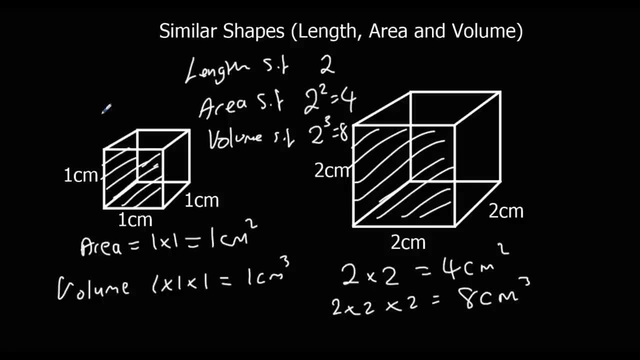 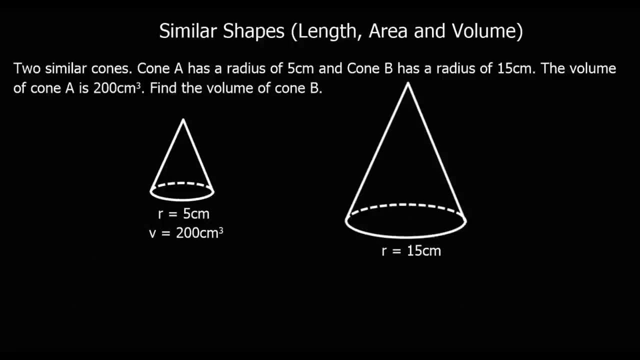 scale factor, you cube it, You cube your normal scale factor, And that's how you are able to work out these questions. So let's have a look at one. We've got two similar cones. Cone A has a radius of 5, and cone B has a radius of 15.. So we 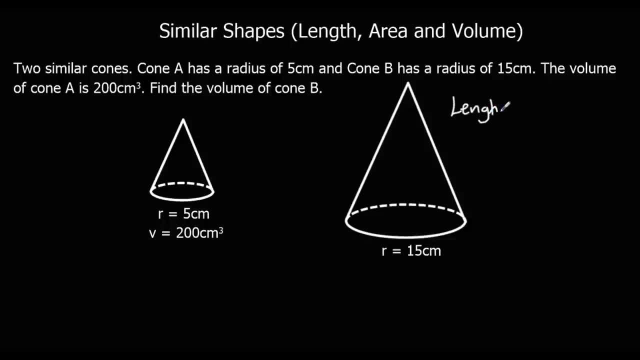 know the length scale factor. the scale factor for length, length scale factor is 15 over 5, which is 3.. So the scale factor for length is 3.. Again, Cone A разeroes 3.. The volume of Cone A is 200.. Work out the volume for Cone B So. 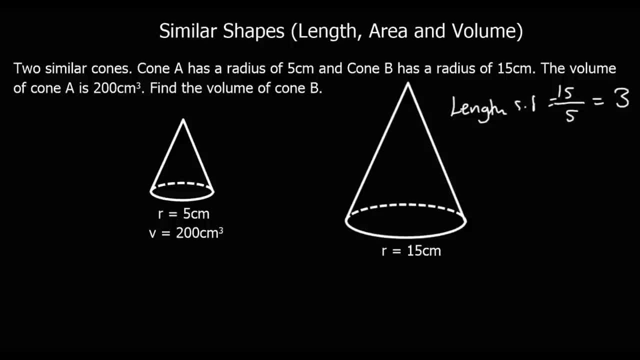 what don't you do is multiply the volume by 3, because that's not the scale factor for volume. The scale factor for volume, volume scale factor, is 3, cubed. So it's volume that's cubed and that is 27.. So what we've got to do to change this volume, we've got. to get the 200.. We've got to multiply by the volume of Cone B and we get B. So that's responding exists and we get b, So the volume per Cone B is not 3.. So then, actually what? I've got here is this: reduce the volume up and I take the 200 and I put it on the scale by the 3 and I multiply. But I don't want to multiply the volume out, So I don't want to multiply. 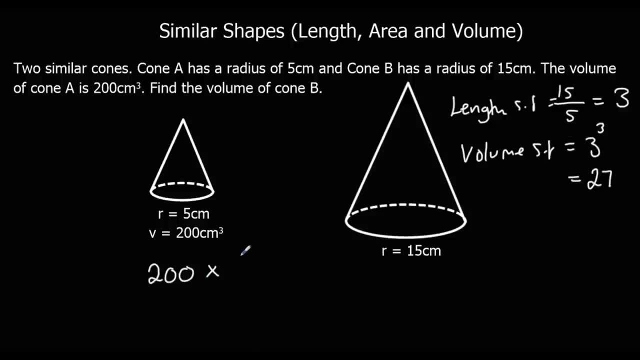 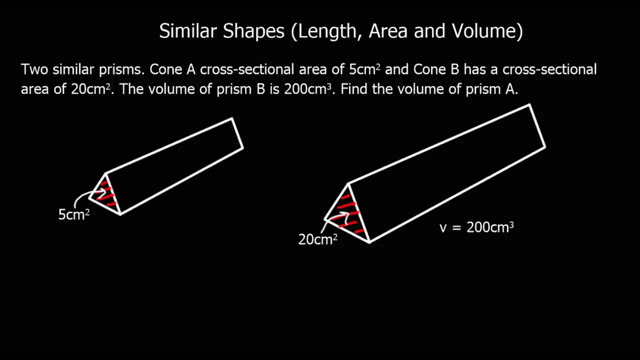 about the volume scale factor, which is 3 cubed, so times 27. so 2 times 27 is 54, and then we add on the two zeros, so we've got 5400 centimeters cubed. okay, now we've got two similar prisms. we've 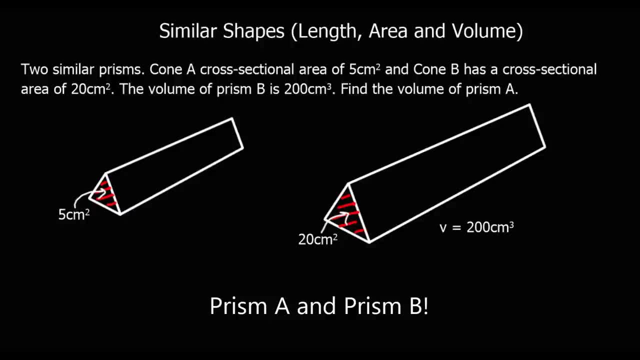 got cone a has got a cross-sectional area of 5 centimeter squared and combi has a cross sectional area of 20 centimeter squared. we've got a workup, we're going to a volume elation, but the first thing we'll do is work at the scale factor, the scale factor for area area. 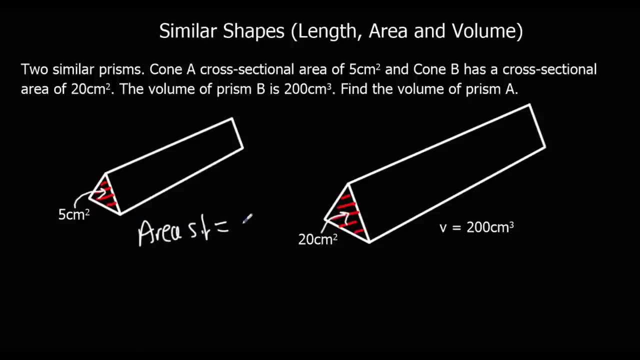 scale factor is 20 over 5, it's 4. so we know the area scale factor. we can't go through the area scale factor. we can't use this, meannox'll just do the same. so it's gonna go as here, to the volume scale factor. The first thing we've got to do is work out the length. 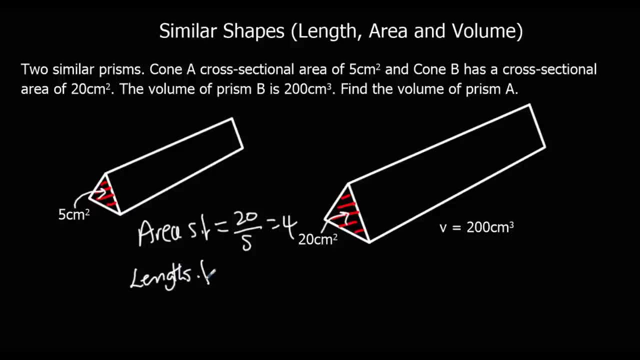 scale factor: Length scale factor. So if the area scale factor is 4, and that's squared, so to find the length scale factor we have to square root it, So the length scale factor must have been 2. And then we can work out the volume scale factor, which is scale factor. 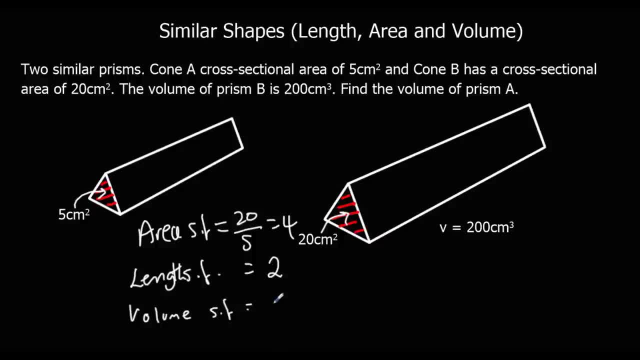 cubed. So this is scale factor squared. We want scale factor cubed 2. cubed is 8.. So we want to go from the big shape to the little shape. So we need to divide by the volume scale factor, which is 8.. So the volume of prison A is 200 divided by 8, which is 100. 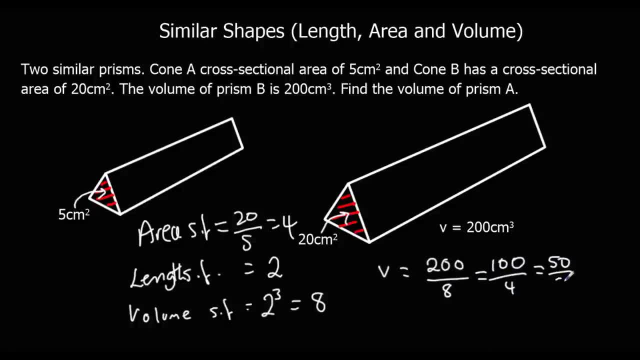 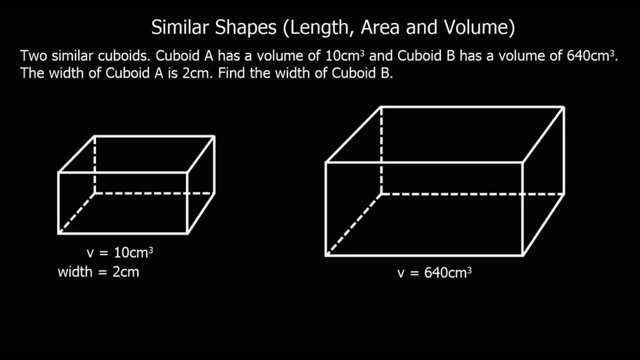 over 4,, which is 50, over 2,, which is 25.. Okay, pause the video and see if you can have a go at this one. So this time we've been given volume, We've been given the small shape with volume of. 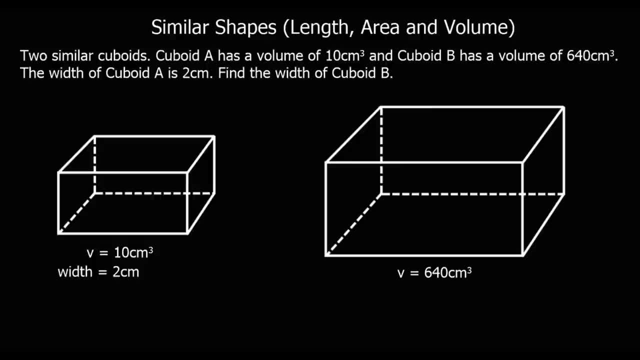 10, and the big shape with a volume of 640.. So we'll work out the volume scale factor first, which would be 640 over 10. Which is 64. But we know that that is scale factor cubed, So to find the length scale. 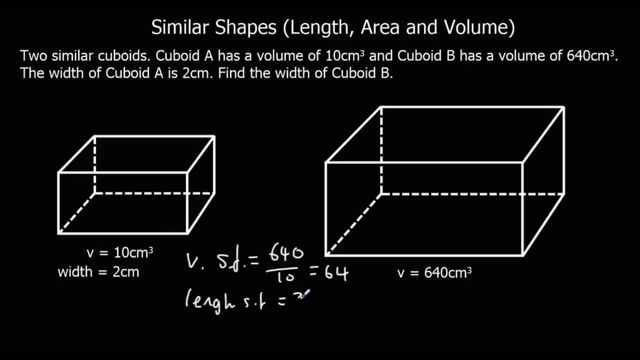 factor- length scale factor- we have to cube root 64. And that will give me 4.. So 4 times 4 times 4 is 64. So the cube root of 64 is 4.. So that's the length scale factor And 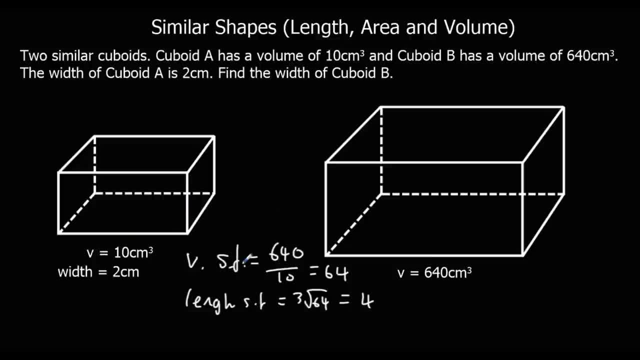 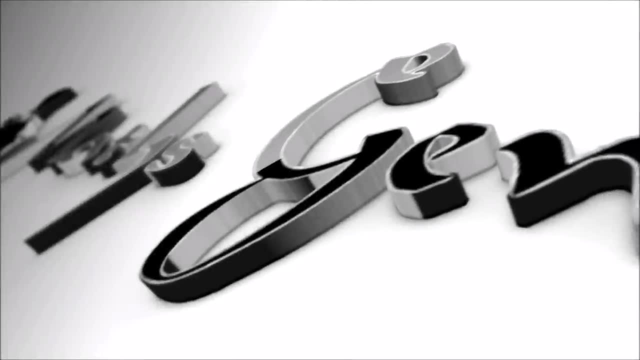 then we need to go from the little shape to big shape. So we're going to times by 4.. So 2 times 4 is 8 centimeters. So the width of cuboid B is 8 centimeters. Thanks for watching and please subscribe for more.